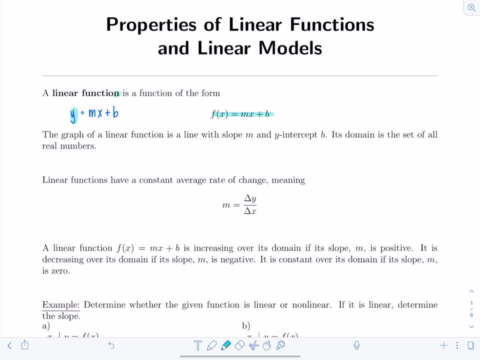 just replacing y with f of x, because we're studying this as a function, now a linear function, and so the graph of a linear function is a line, the slope is equal to m and the y-intercept is b or zero comma b. The domain is the set of all real numbers. you can substitute in any number for x. 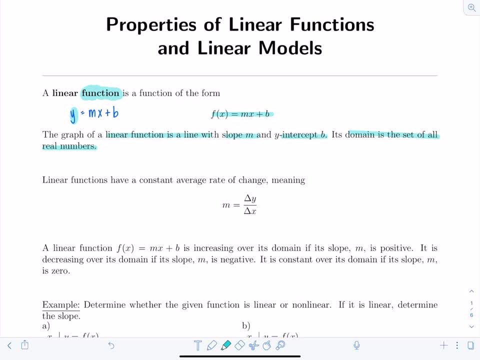 our function is going to be defined Now. linear functions have a constant average rate of change because they have a constant slope. So the slope is equal to the change in y divided by the change in x, and this quantity here represents your average rate of change. change in y over change. 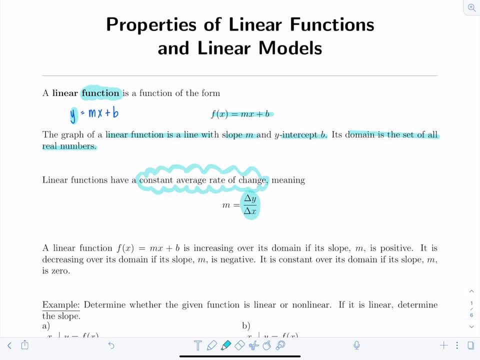 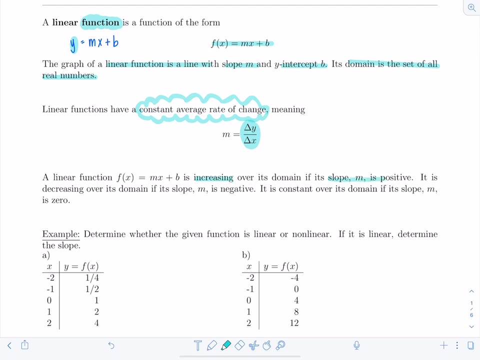 in x and linear functions are special because that ratio remains constant throughout the entire graph for the whole function. Now we say a linear function, f of x is increasing over its domain if its slope m is positive. Basically, if you were to walk on the linear function from left, 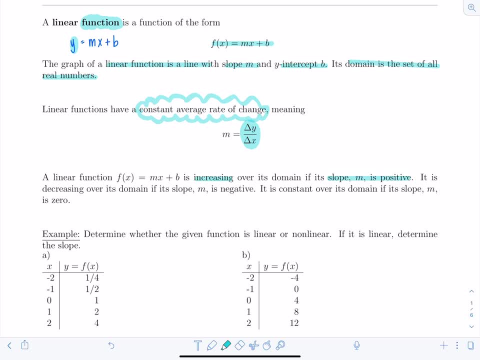 to right. you'd be going uphill the whole time. and then it's decreasing over its domain. if the slope is negative, The linear function is constant over its domain if the slope is zero. if you have a horizontal line, Okay, and then notice we don't talk about vertical lines because they're not. 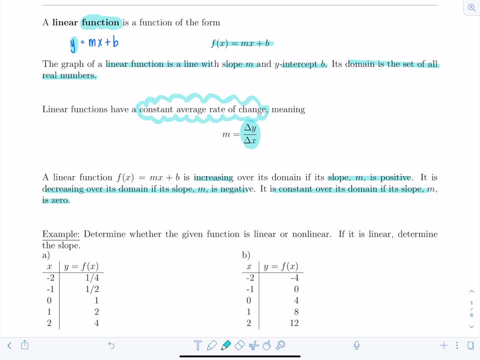 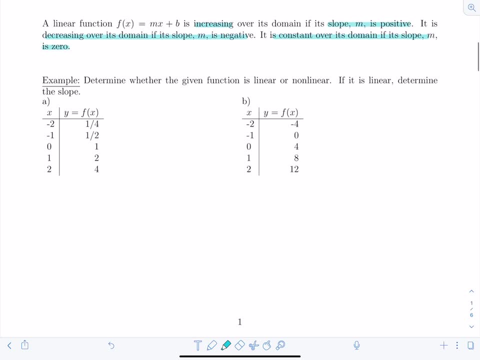 functions, they don't pass the vertical line test. We're only studying linear functions right now. All right. so first example here: determine whether the given function is linear or nonlinear and if it's linear, determine the slope. So, in order to test, since they don't give us the equation for f of x, what I need to do is look at what the average 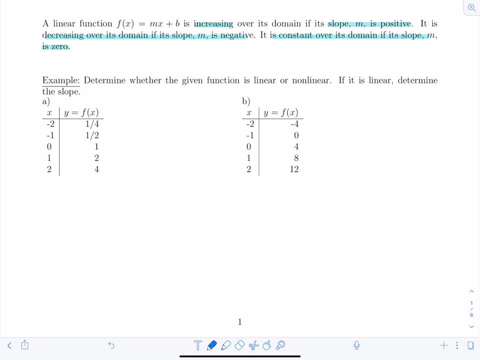 rate of change is, and I need to have a constant average rate of change, meaning the change in y divided by the change in x would be constant. So notice here: the change in x is always one right. we're going up by one in the table, and now let's. 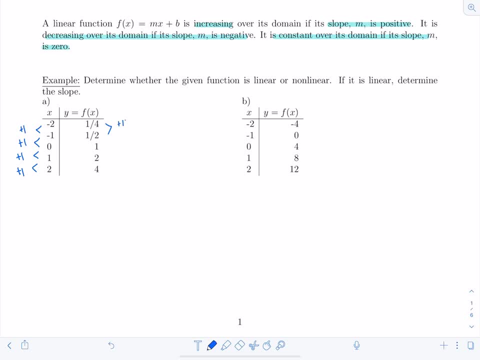 look at the change in y. So, from one-fourth to one-half, we added a fourth. from one-half to one, we added a half. now we added one. now we added two. So the change in y is not constant. the change in x is constant here on the table, but not the change in y that corresponds with it. So no, this is not. 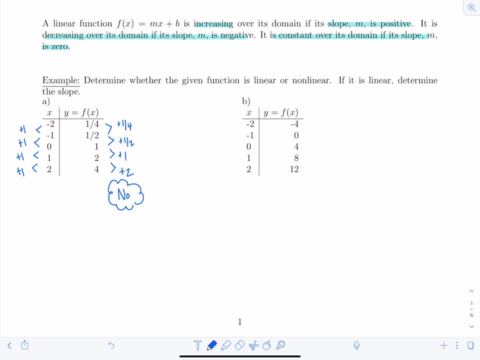 a linear function. What about example b? So again, the change in x is constant. we're just adding one. So change in x is one. Now what about the change in y? So from negative four to zero, we added four. Same here: four to eight, you add four. eight to twelve, you add four. So it looks like the change in y. 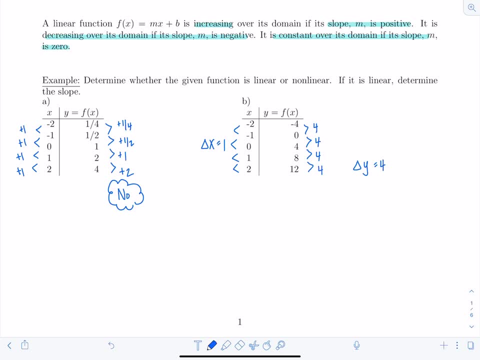 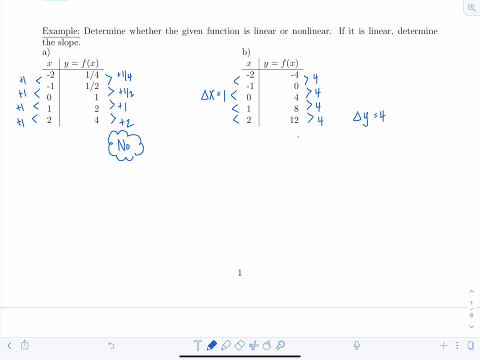 is equal to four for all the values that we were given. All right, so this given function looks like it's linear. so we're gonna say yes, and now we need to find the slope. Well, remember, the slope is the change in y over the change in x, and we found the change in y. 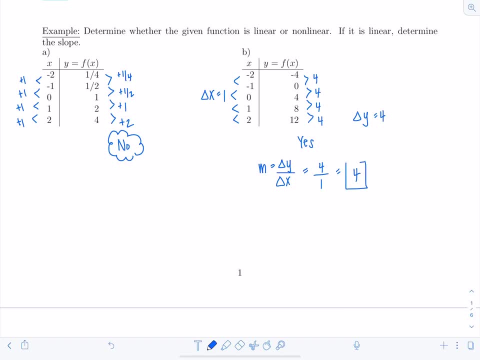 to be four. change in x is one, so the slope is four. All right, that's equivalent to taking two ordered pairs like negative, two negative, four. right, they go together. And then another two ordered pairs like negative, one zero. and then you could still use: M is y two minus y one over x, two minus x one. but it didn't do it that. 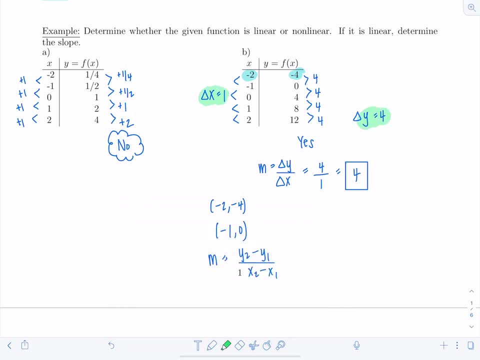 way, because we already looked at the change in x and the change in y from the table to decide whether it was linear or not to begin with. So it was just easier to do it that way and find the slope. But you could still do it the way maybe you're used to from before. 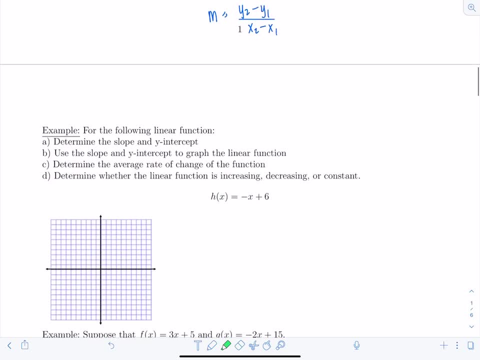 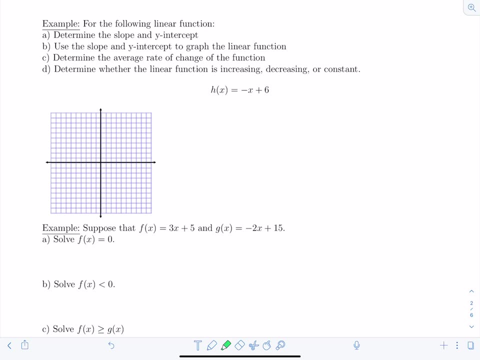 All right, moving on For the following linear function. so now we know for sure we're working with the linear function. we're going to determine what the slope and y-intercept are and then use the slope and y-intercept to graph determine the average rate of change of the. 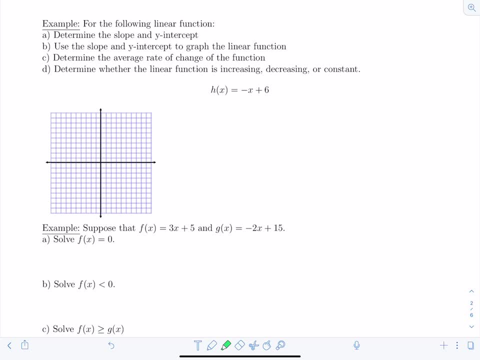 function and then determine whether it's increasing, decreasing or constant. So here's our linear function: h of x equals negative x plus 6.. All right, so let's get started. First thing we need to state is the slope and y-intercept. So slope, that's the coefficient. 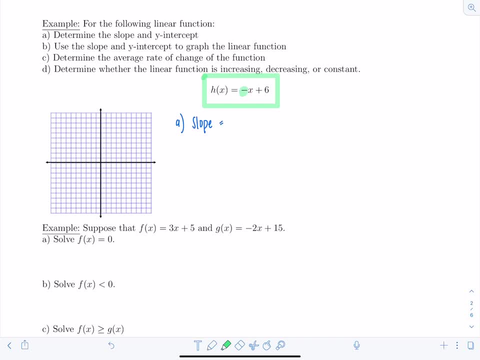 on x. so the slope is negative 1, and the y-intercept is 6, but remember always write it as an ordered pair. so 0, 6.. Very good, Now we're going to use the slope and y-intercept. 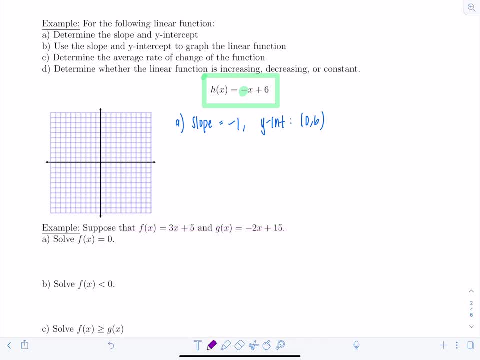 to graph the linear function. So the y-intercept is at 0, 6.. Let's label our axes: Here's x, here's y. I'm going to go up 6 on the y-axis, so 1,, 2,, 3,, 4,, 5,, 6, and then the slope is. 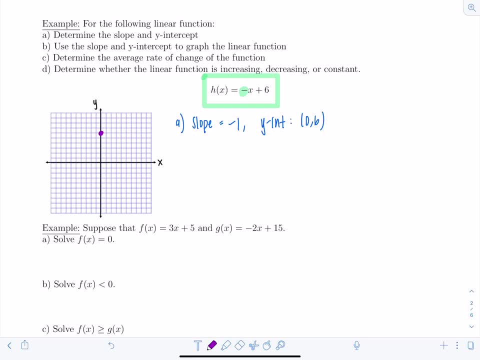 negative: 1.. So I could go down 1,, 1 to the right, or I'm going to be really slick and go down 6 and then go 6 to the right: 1, 2,, 3, 4, 5, 6.. That way my line will look a little. 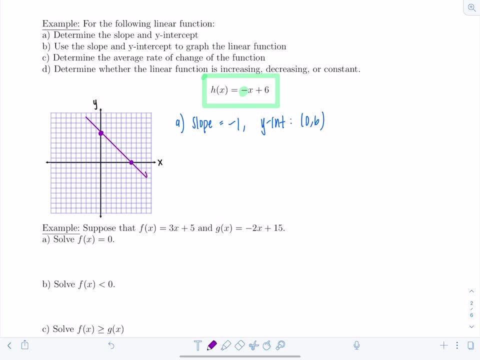 bit nicer. And there we go. Don't forget the arrows. All right, so part A is done, part B is done. Determine the average rate of change. Remember, the average rate of change is equal to change in y over change in x, and for a linear function that's just equal to the slope which we already 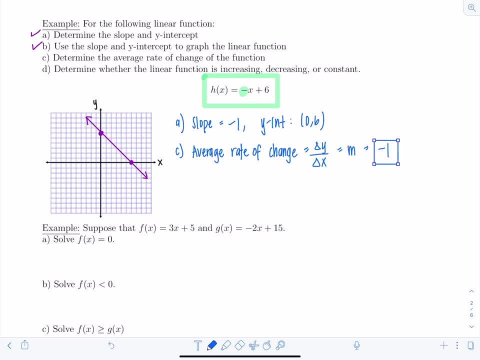 have It's negative 1.. Okay, not bad. And then last determine whether the linear function is increasing, decreasing or constant. So you just have to look at the slope. Since the slope is negative 1, which is less than 0, that means it's decreasing, And you can just imagine if you were to walk. 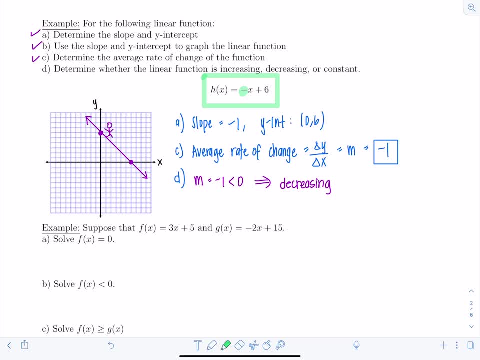 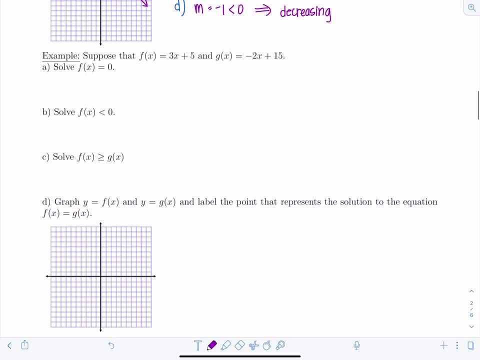 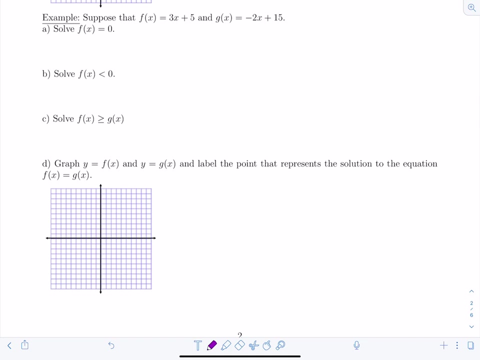 on this graph from left to right, so you always go in that direction. Whee, You're going downhill. So it's decreasing Beautiful, All right. next example, a little something different. So suppose f of x is equal to 3x plus 5 and g of x equals negative 2x plus 15.. So part: 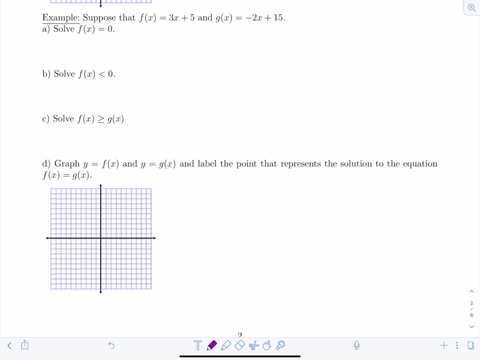 A asks us to solve: f of x is equal to 0. So they're telling me to set the function, in this case 3x plus 5, equal to 0. So I'm going to do that. So I'm going to do that, And then 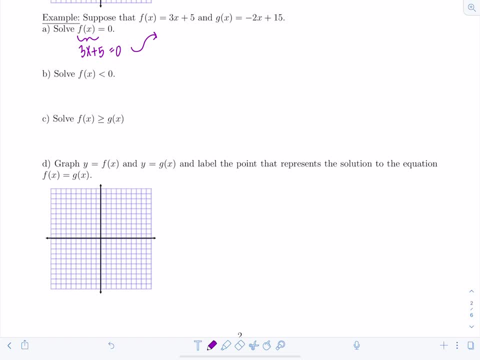 I'm going to solve: f of x is equal to 0 and solve So. if I solve, that means 3x is equal to negative 5 or x equals negative 5 thirds. All right, not bad. Now solve: f of x is less. 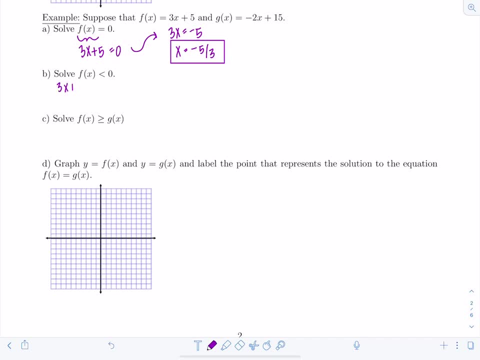 than 0.. All right, so I'm going to take the function 3x plus 5, set it strictly less than 0. That means 3x would be less than negative 5.. So x would be less than negative 5 thirds. 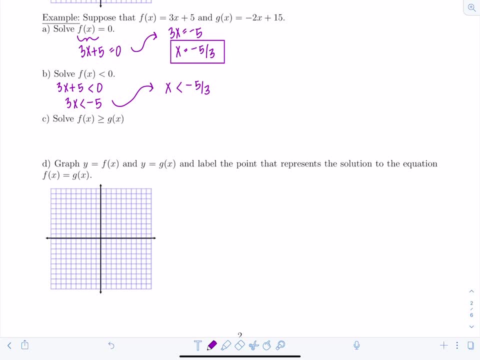 All right, you could leave it like that, or an interval notation: If x is less than negative 5 thirds, that would be the interval from negative infinity until negative 5 thirds, and then put parentheses, since we're not including negative 5 thirds. Other option, if you write: 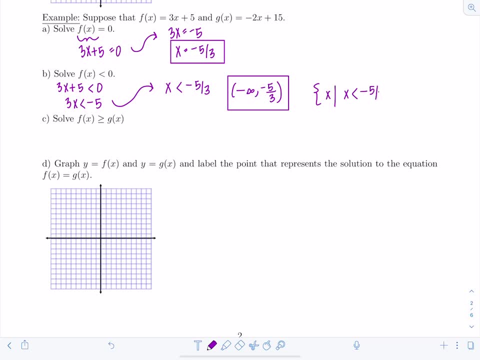 it in set builder. you'd say x, such that x is less than negative 5 thirds. Okay, last one Solve: f of x is greater than or equal to g of x. So we're going to set 3x plus 5 greater than or equal to g of x. What was g of x? It was: 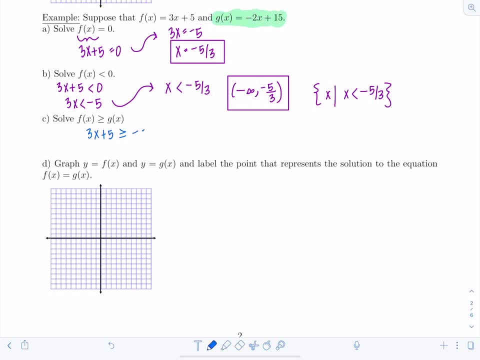 right here: negative 2x plus 15.. So let's get all the variables together. I'm going to add 2x over to the other side. Let's subtract 5 while we're at it. Dividing by 5, now I get. 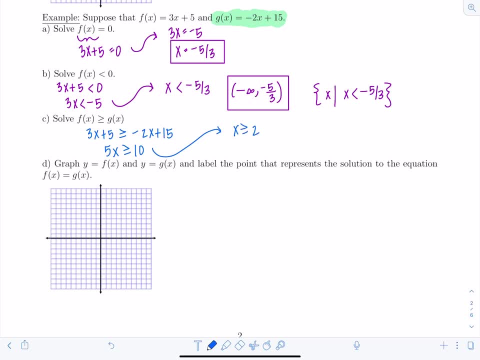 x is greater than or equal to 2.. Okay, an interval notation: x greater than or equal to 2, you would include 2. This time. so I'm going to put a bracket up until positive infinity always. parentheses on infinity, always, always. Okay, if you want to write that in set builder, then you. 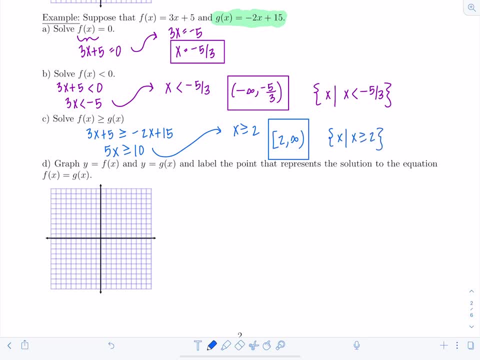 would say x, such that x is greater than or equal to 2.. Lovely, All right, and now we're going to graph them. So we're going to graph y equals f of x and y equals g of x on the same coordinate axes, Okay, and then label the point that's. 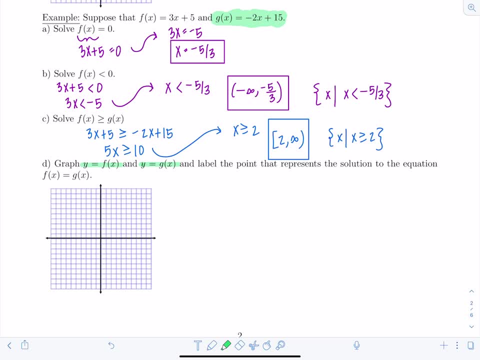 right here: negative 2 and plus x greater than or equal to 2.. An integral function f of x is greater than or equal to 2.. We're going to write this one and then replace the single points. So we're going to write this one and then replace the single points. 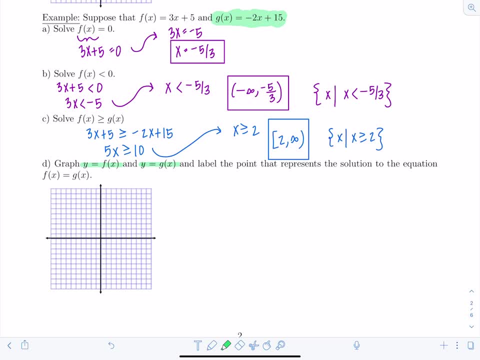 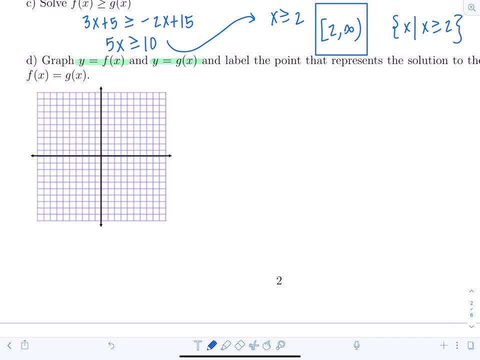 So that represents the solution to the equation f of x equals g of x, where they equal each other. Okay, so let's go ahead and get started. I'm going to write down the functions first. So f of x is equal to 3x plus 5.. So that means the slope is 3 and the y-intercept is: 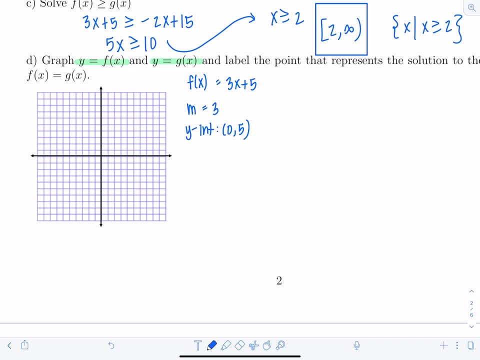 0, 5.. So I'll plot that at the y-intercept 1,, 2,, 3,, 4,, 5, and then you can go up 3, over 1, up 3, over 1,, so on and so forth. 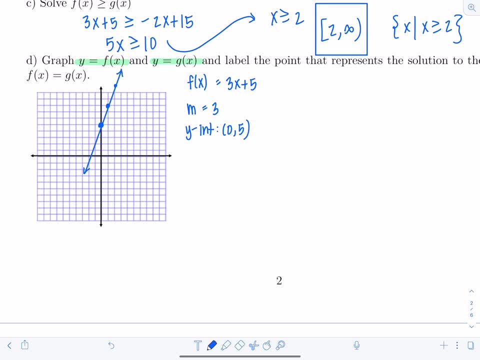 So there's f of x and then g of x. g of x's equation was negative: 2x plus 15.. Oh, I can't fit 15 on there, Anyways, let's just use something else. I know the slope is negative. 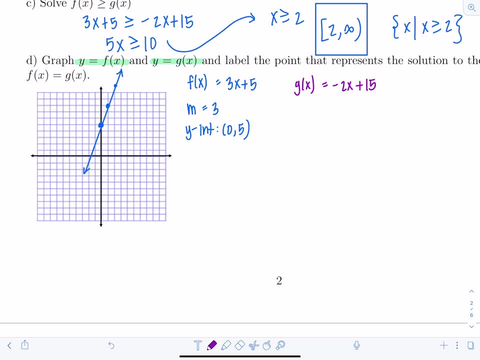 2, so I can plug in a different point if I want. Say, I plug in 3,. so g of 3 is going to be negative 2 times 3 plus 15,, that's 6 plus 15,, which is 9.. So I have 1,, 2, 3, 1, 2,, 3,, 4,, 5, 6, 7,, 8, 9,. 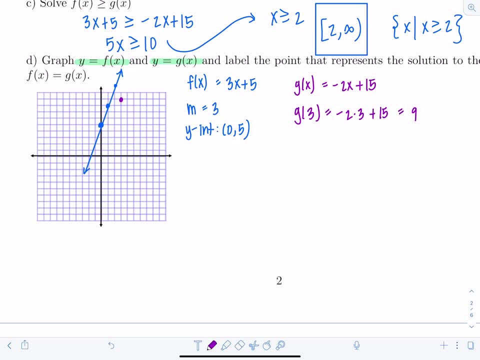 right here, and then the slope is negative 2, so from there I can go down 2, 1 to the right, or I could go up 2, 1 to the left. That's enough. So there's g of x and there is f of x right there. 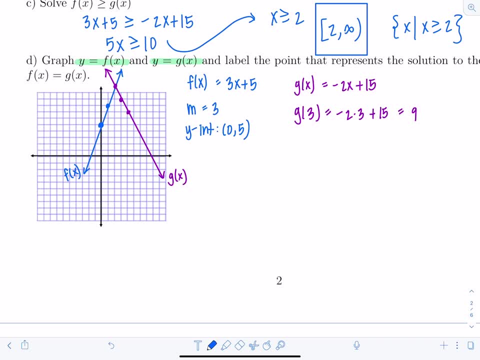 Now they're asking us to label the point that represents the solution to the equation. f of x equals g of x. So the solution to the equation is going to be where those two graphs meet or intersect. Can you see where that happens? It's right here.